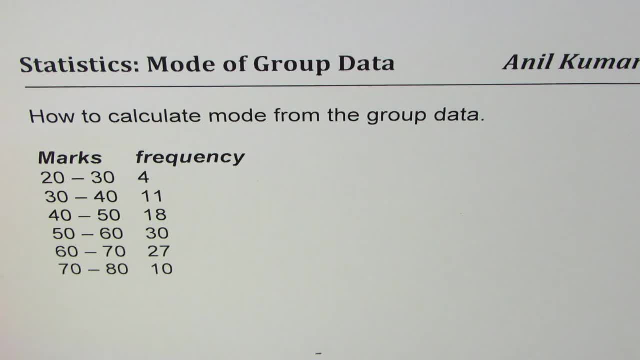 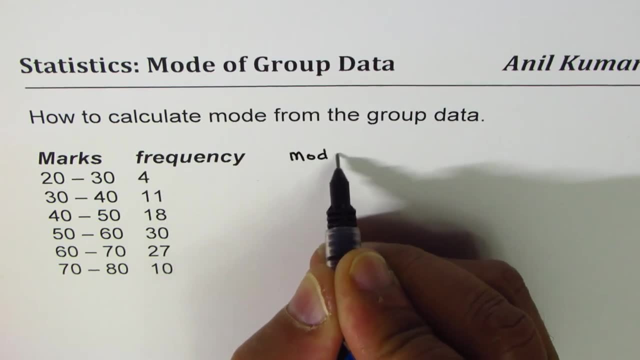 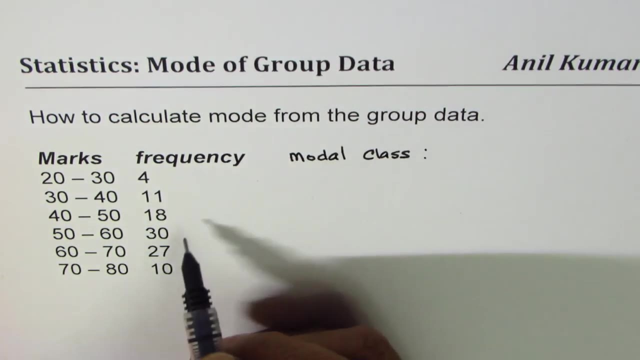 Mode, as you know, is most frequent When we are dealing with group data. we actually first try to find what is the modal class? right? What is the modal class Now? modal class is the class where we have highest frequency, is that right? So modal class will have the highest frequency of the group. 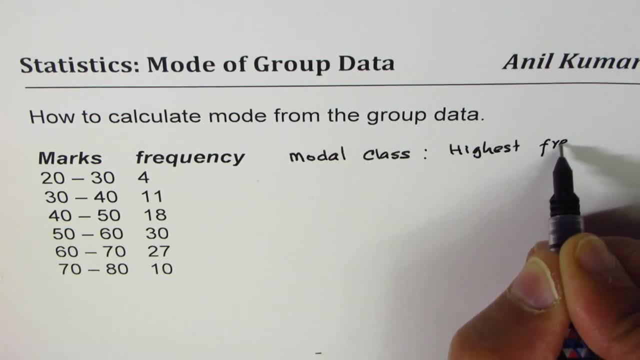 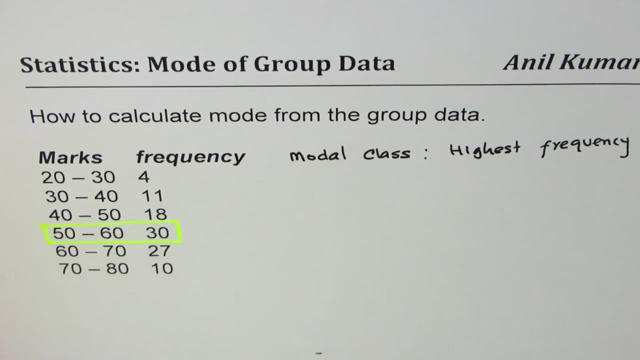 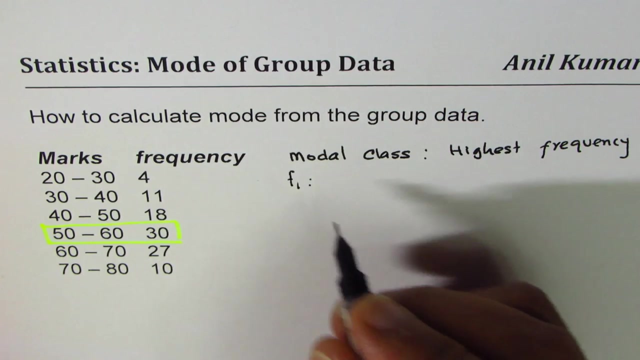 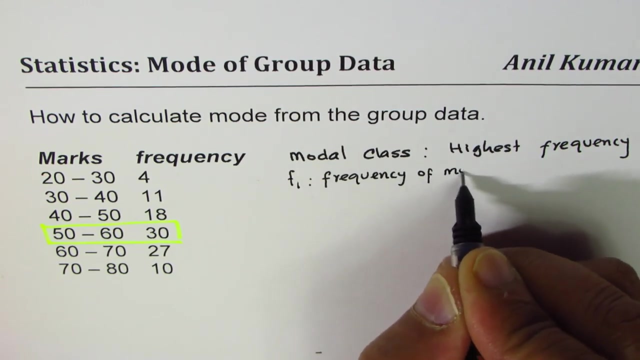 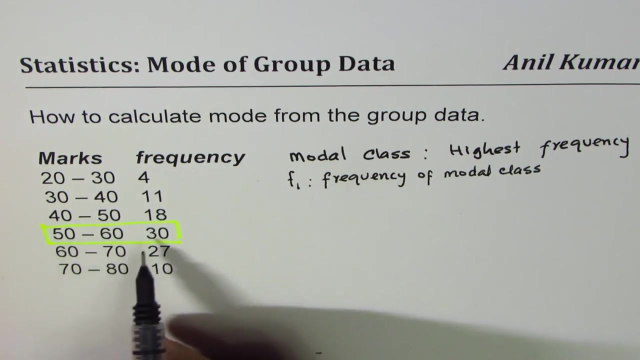 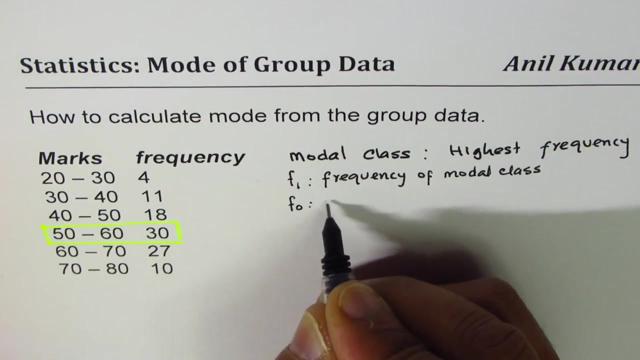 highest frequency. so in our case 30 is highest in the frequency. so the model class is 50 to 60. correct this frequency. we call this as f1. right, so we'll call this as f1. f1 is the frequency of mode of class. now the frequency which is before the mode class will call this as f0, which is: 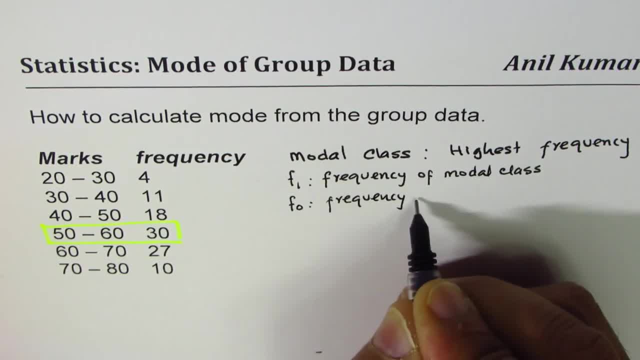 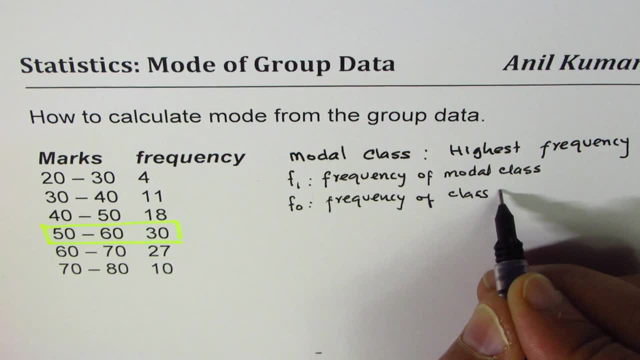 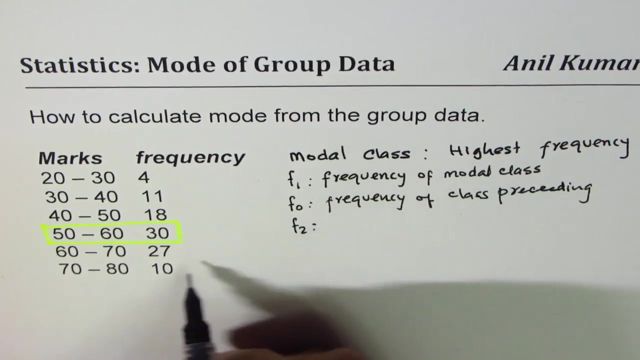 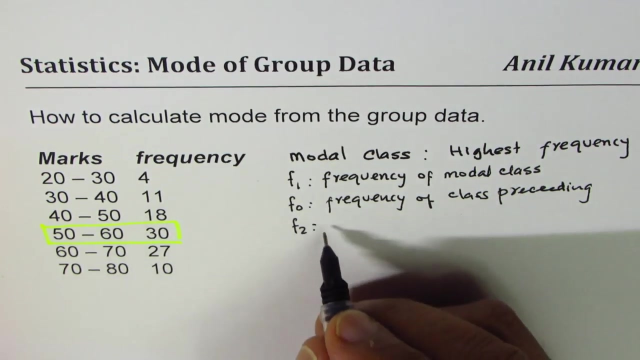 frequency of class. we could call it preceding class, right, so we'll call class which comes before, so class which is preceding. we'll also deal with the frequency f2, which is frequency of the class preceding the or following or succeeding the model class. so we'll call f2 as frequency. 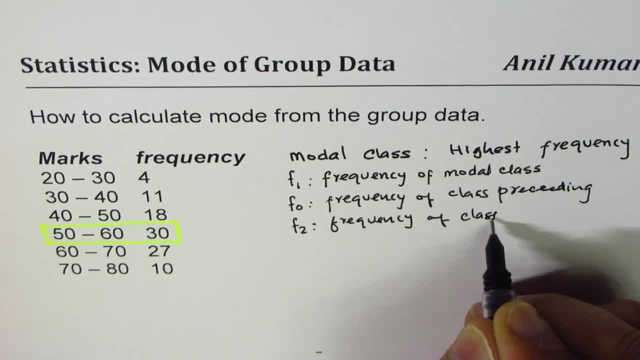 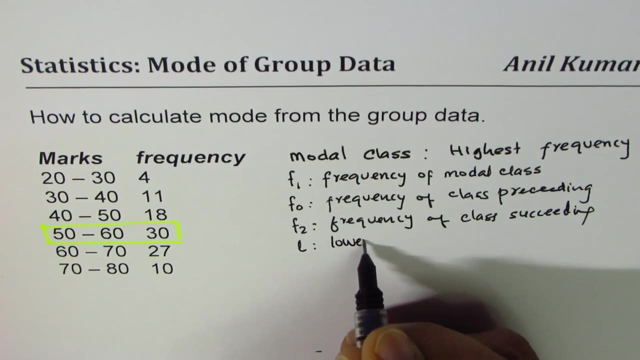 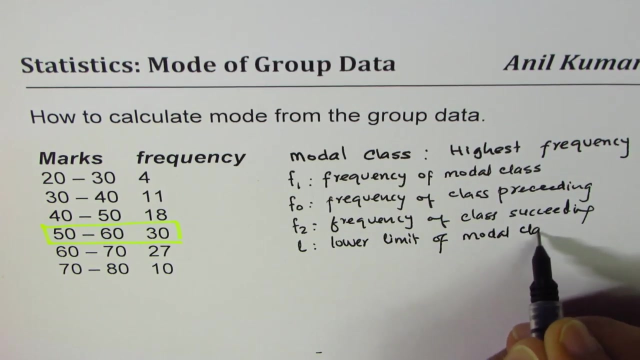 of class succeeding. I should have written succeeding class and preceding class. anyway, we'll use this lower limit of mode class will write L for this lower limit of model class and the class interval. so let me use the simple h for class interval mode is given by the former. let 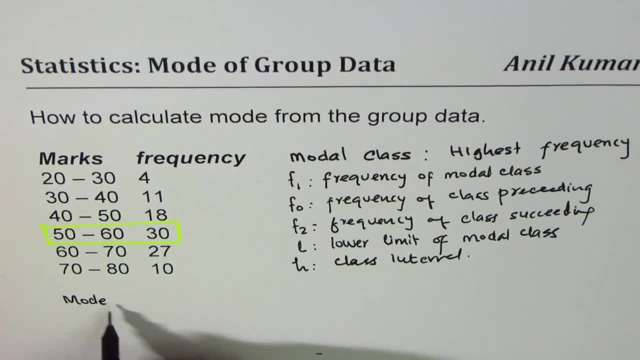 me write down the former for mode. mode is equal to L, the lower limit of the model class plus frequency of model class, which is f1 minus frequency of the preceding class, which is- we'll put a symbol- F0, for now, divided by two times model class frequency. take away F0 and F2, where F2 is the frequency of succeeding. 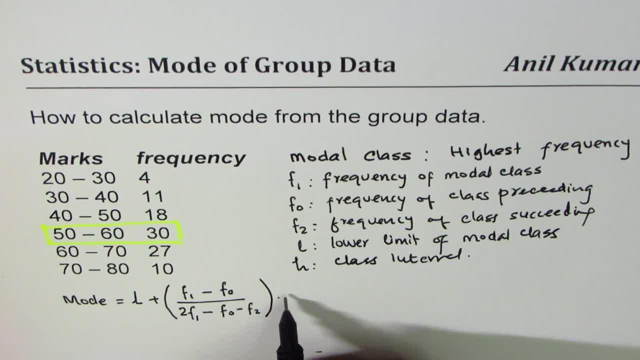 class right times H. So that is the formula which you can use to find or calculate the mode. Remember, this is just an estimate. So L, in our case, is what We can see from here. L is 50,. right, Let me write down the values here. L is 50.. Let's start from here. 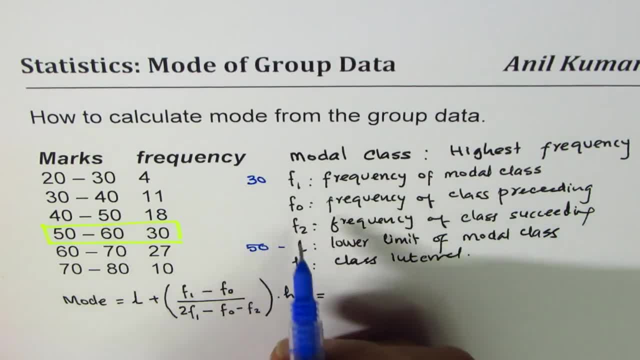 Frequency for the model class is 30,. correct F0 frequency before that is 18.. The frequency after model class is 27.. The class interval is 70 minus 60 or 60 minus 50, which is 10.. Substituting these values and calculating: 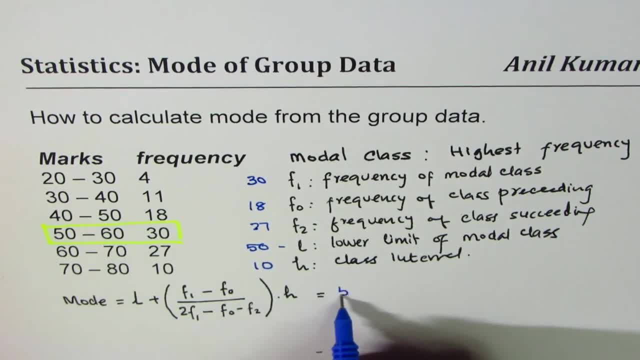 we should get more right. So we'll write 50 plus within brackets. F1 is 30. Take away 18, divided by 2 times 30, right. Take away 18 and 27.. and multiply this by age, which is 10, correct, so that should give you the. 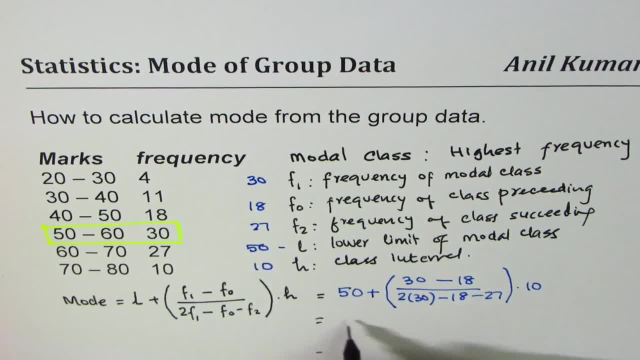 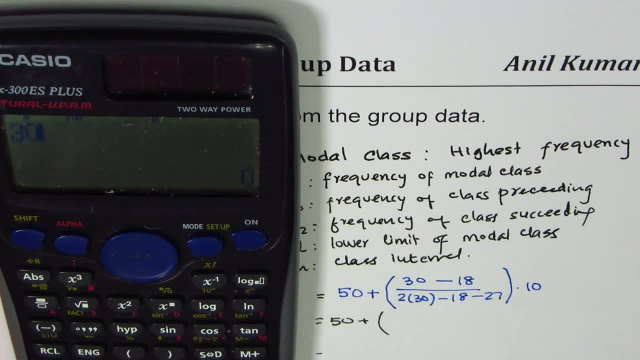 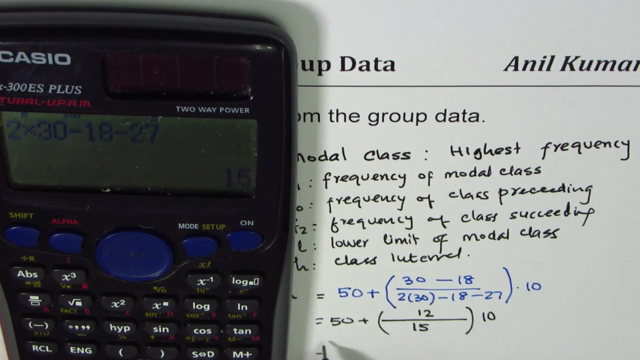 answer, which is: let's write down 50 plus. let's use the calculator: 30 minus 18 equals to 12 divided by 2 times 30. take away 80, take away 27, that gives us 15 times 10. right, so that gives us equal to 50 plus. so let's say 120 divided by 15.